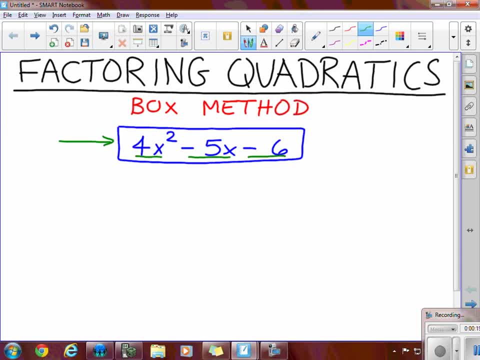 I have a 4x squared, a negative 5x and a minus 6.. None of the numbers 4,, 5, or 6, have any common factors, and the first two terms have x's in them. The last one does not. 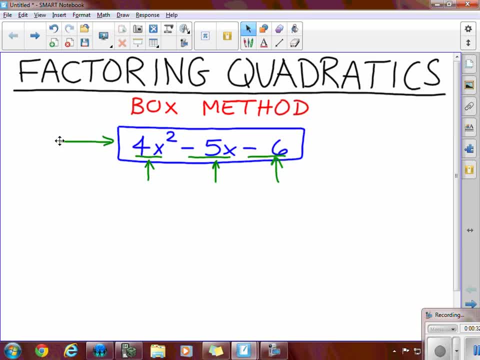 so there is no variable that's similar between them, so there is no greatest common factor in this example. So now we just have to look at putting this in the box. So the box method means I create this box and in this box two things have to happen. This first term: 4x squared. 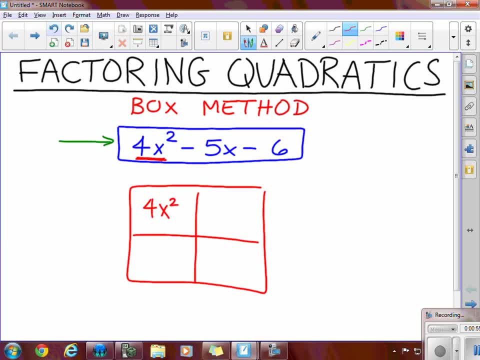 has to go in the top left corner. The last term, the constant, goes in the top left corner. So I create this box, and in this box two things have to happen: The bottom right corner. So that's how we set up the box to begin with. Now the next step. 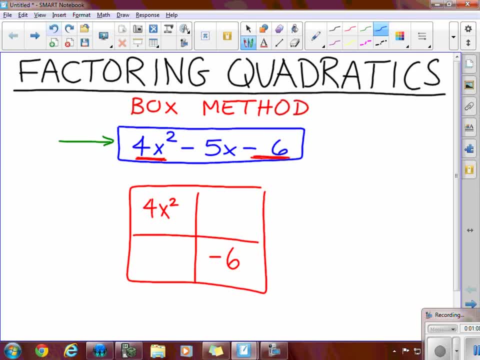 is to do a little bit of math to figure out what we're actually looking for. We need to find two sets of numbers. These two sets of numbers have to multiply to something and they have to add to something. So to figure out what these two sets of numbers have to multiply to, 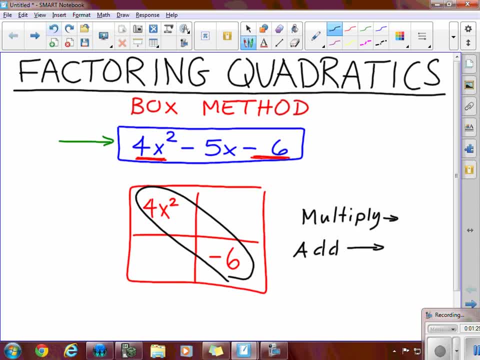 we just look at these two numbers. What is 4x squared multiplied by negative 6?? So 4x squared multiplied by negative 6 is negative 24x squared, The add to part. we need to find two terms that add to the middle term in this quadratic. 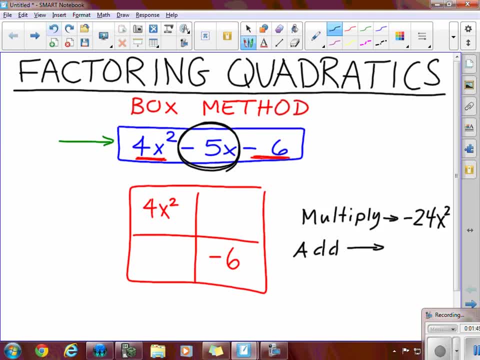 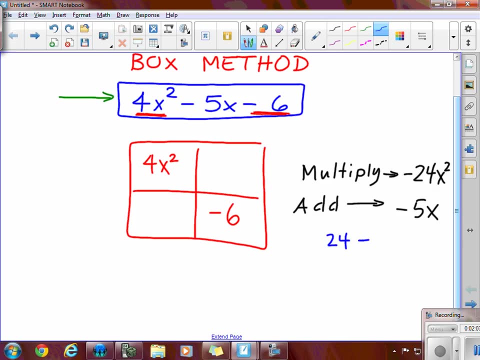 So we need two things that will add to a negative 5.. So it has to add to a negative 5x. Now, one of the easiest things to do is to look at what we're trying to find something to multiply to. So I'm trying to find 24.. There's only a limited number. 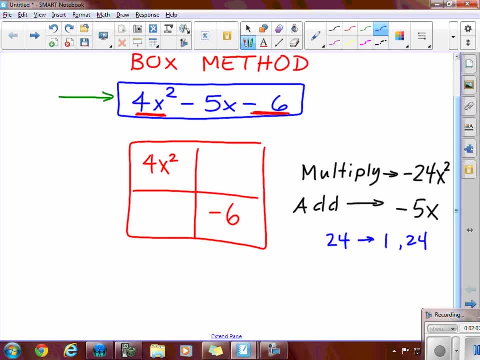 factors of 24.. We have 1 and 24.. We have 2 and 12.. We have 3 and 8. And we have 4 and 6.. Those are the only four sets of numbers that will actually multiply to a 24. So now we look at these sets of. 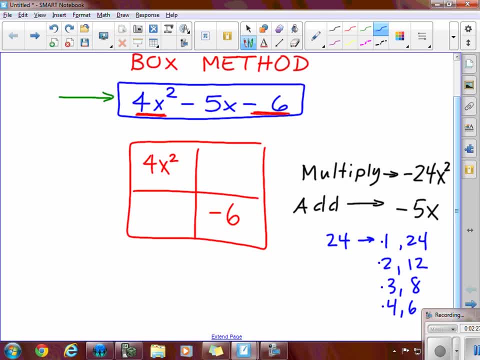 numbers and we try to say which one of those would somehow produce a value of 5? Well, 1 and 24 won't, 2 and 12 won't, But 3 and 8, there is a difference of 5 between them. 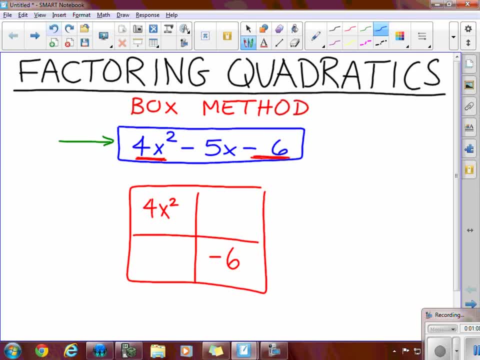 is to do a little bit of math to figure out what we're actually looking for. We need to find two sets of numbers. These two sets of numbers have to multiply to something and they have to add to something. So to figure out what these two sets of numbers have to multiply to, 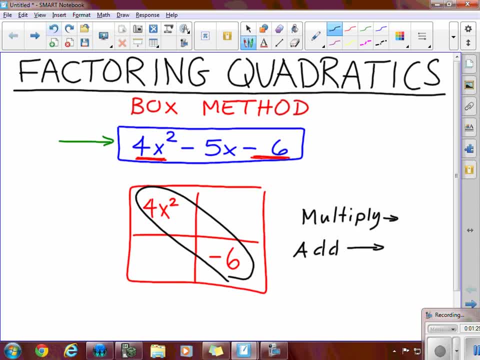 we just look at these two numbers. What is 4x squared multiplied by negative 6?? So 4x squared multiplied by negative 6 is negative 24x squared, The add to part. we need to find two terms that add to the middle term in this quadratic. 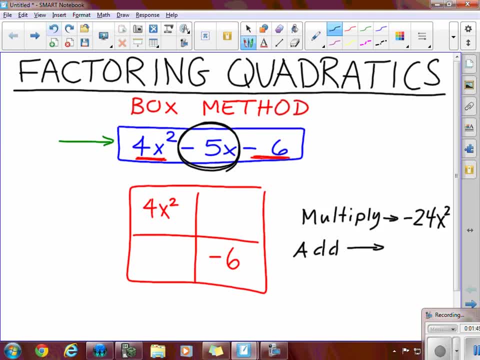 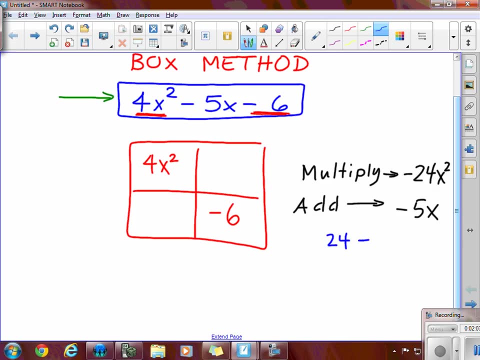 So we need two things that will add to a negative 5.. So it has to add to a negative 5x. Now, one of the easiest things to do is to look at what we're trying to find something to multiply to. So I'm trying to find 24.. There's only a limited number. 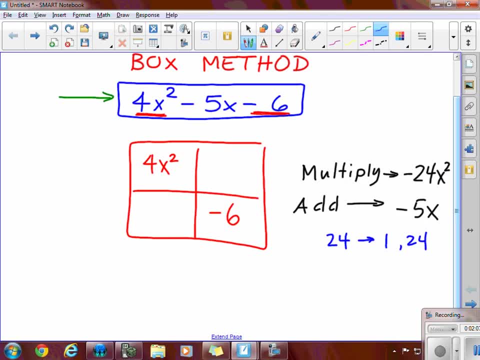 of factors of 24.. We have 1 and 24.. We have 2 and 12.. We have 3 and 8. And we have 4 and 6.. Those are the only four sets of numbers that will actually multiply to a 24.. So now we look at these. 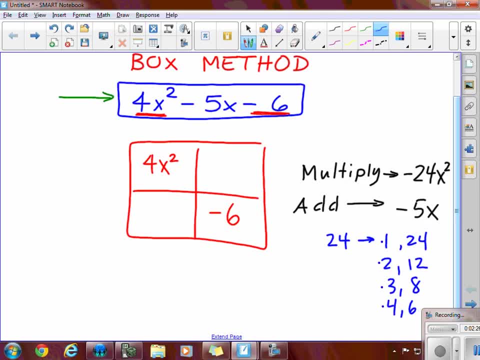 sets of numbers and we try to say which one of those would somehow produce a value of 5? Well, 1 and 24 won't, 2 and 12 won't, But 3 and 8, there is a difference of 5 between them. 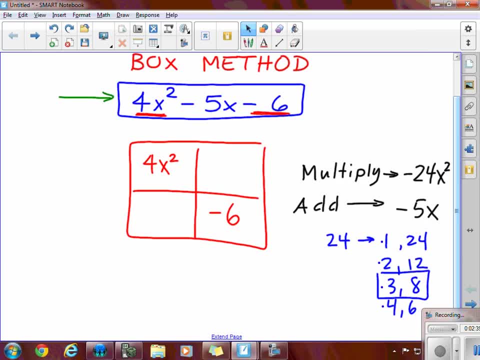 So my two numbers that I'm going to use are a 3 and an 8, with some x's here. Now remember that these two terms have to add up to a negative 5x. So to add to a negative 5x, the 8 term has to be: 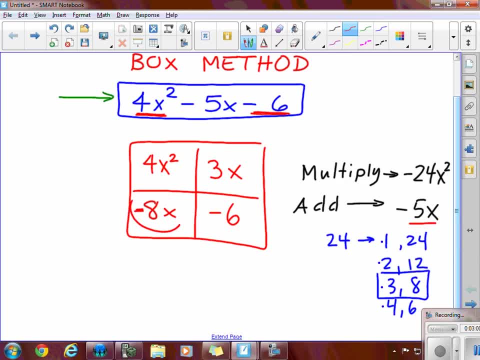 negative 8x, Because If we look, negative 8x and 3x add to a 5x And negative 8x and a 3x multiply to a negative 24x squared. So those are the two terms that we need to use Now. the last step in the box method is: 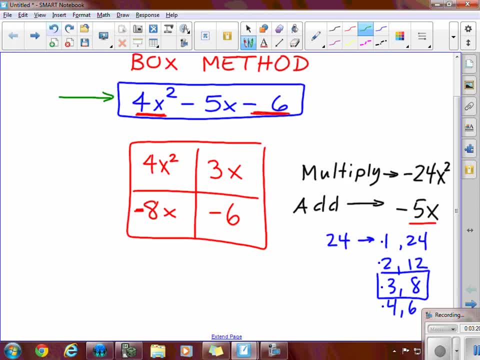 to look at individual rows and columns in the box and take out greatest common factors. So in this first row, if I looked at these two numbers, the biggest thing that I could factor out of both of is simply an x. If I look at the next column, or sorry, the next row, the biggest thing I can 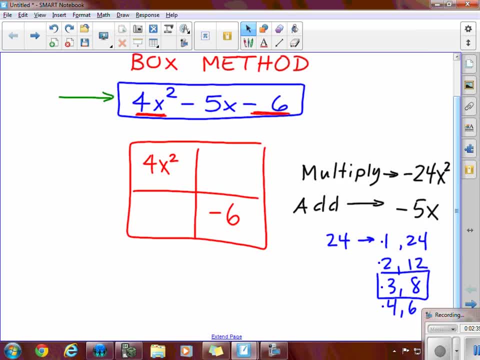 So my two numbers that I'm going to use are a 3 and an 8, with some x's here. Now remember that these two terms have to add up to a negative 5x. So to add to a negative 5x, the 8 term has to be: 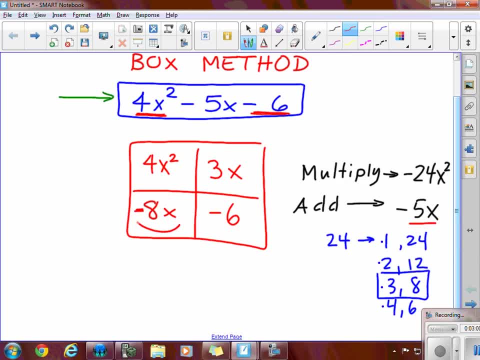 negative 8x, Because if we look, negative 8x and 3x add to a 5x And negative 8x and a 3x multiply to a negative 24x squared. So those are the two terms that we need to use Now. the last step in the box method is: 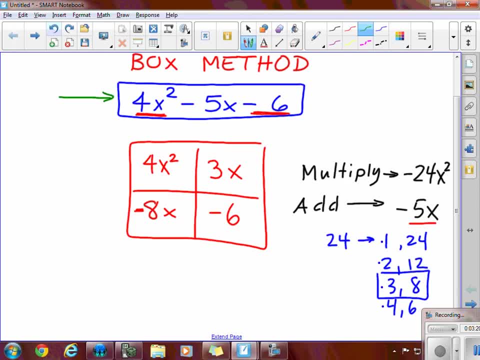 to look at individual rows and columns in the box and take out greatest common factors. So in this first row, if I looked at these two numbers, the biggest thing that I could factor out of both of is simply an x. If I look at the next column, or sorry, the next row, the biggest thing I can factor 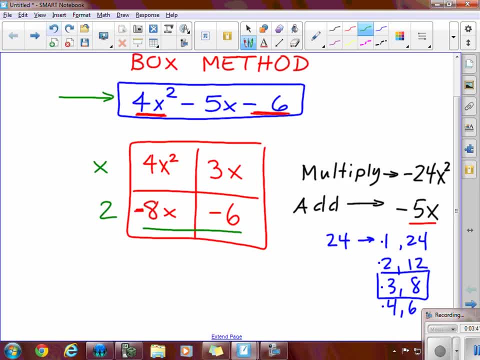 out of both of those is a 2.. If I look at the first column, I have a 4x squared and a negative 8x. The biggest thing I could factor out of both of those is a 4x, And the last column, I have a 3x. 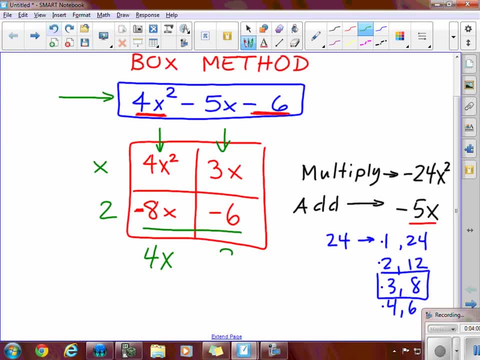 and I have a 6. The biggest thing I could factor out of there is 3.. But now inside my box some numbers are negative. So that means either this 2 term or this 3 term has to be negative. And in order to do it, we just say: 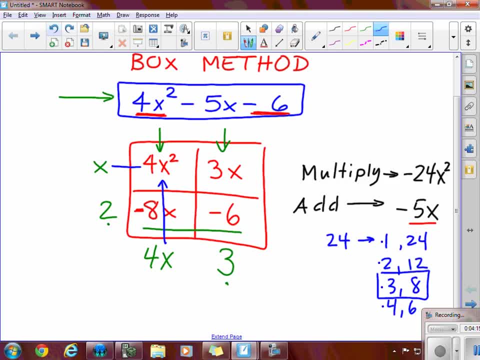 look at the chart and we say 4x times x, That's a positive 4x squared. So that's good. If I look here, 4x times 2 does not give me a negative 8x. So what I do is make that constant term a negative And I continue doing the same process, saying x times 3.. 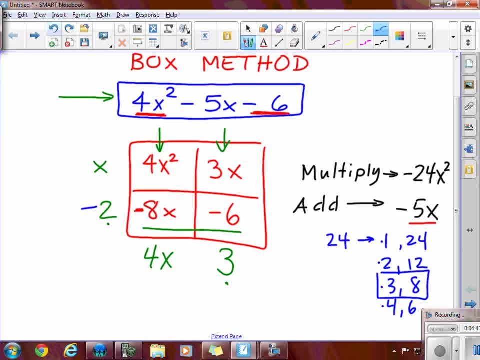 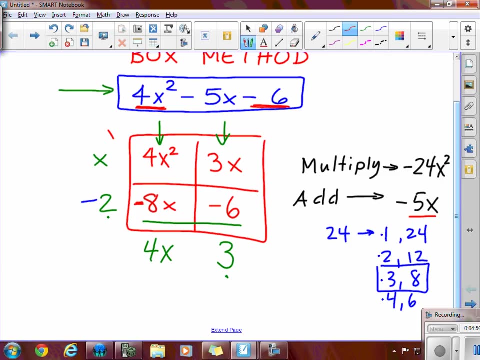 Well, that's positive 3x, so that works. And now I have negative 2 times a positive 3. That's negative 6. So the negative is on the right term. Now my quadratic is simply factored. Here is one factor.